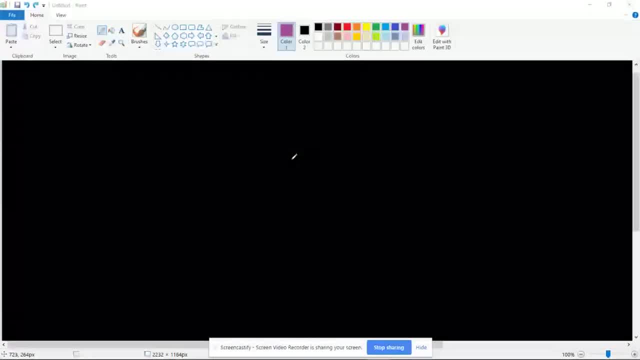 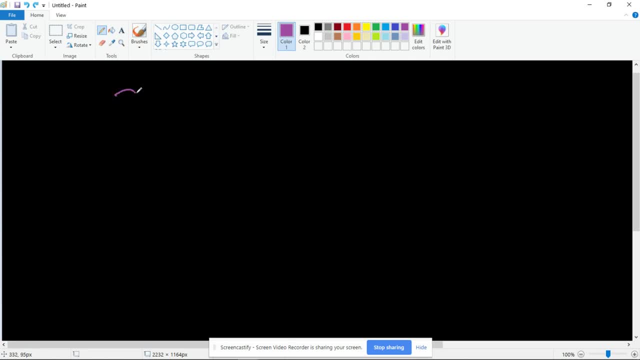 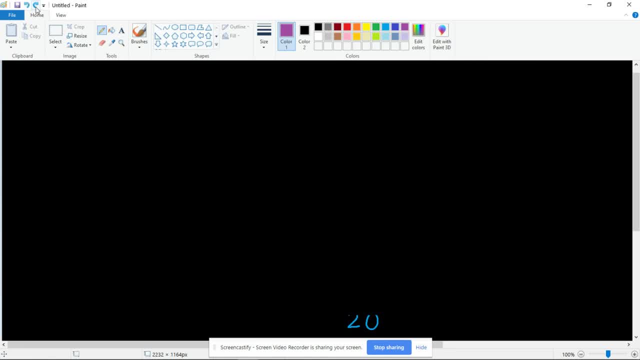 an answer like that on a calculator or something similar. So let's quickly just make one up here. Let's go three into 11.. So we're taking the number 11, divided by three. Let's move this right up to the top so we have room to work. Okay, we're going to skip this step because in the 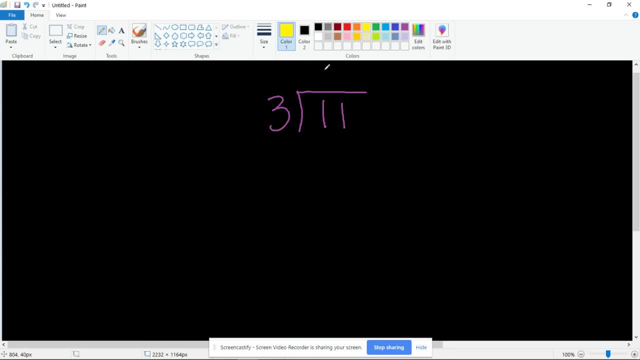 previous video I showed you what to do. doing how many times is three going to one? it doesn't. So we did: zero times three is zero, minus sign one down there. just drop the one down, We're still at 11.. So we're going to skip that step in here. Show you a little trick: How many times is three? 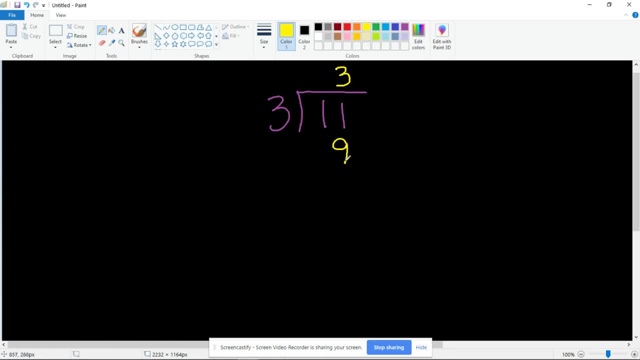 going to 11?? It goes three times. Three times three is nine. 11 minus nine is two. Let's change the color here. Let's go something really bright. Let's go red. Put the zero in there, Put your decimal in. 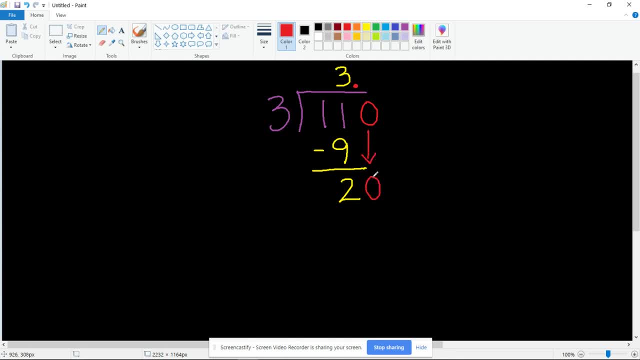 like I said in my previous video, Drop the zero down 20.. How many times is three going to 20?? The answer would be six. Six times three is 18.. And watch what happens here. We get another two here. If I put a zero here again, we drop it down. It's going to be another 20.. Just, 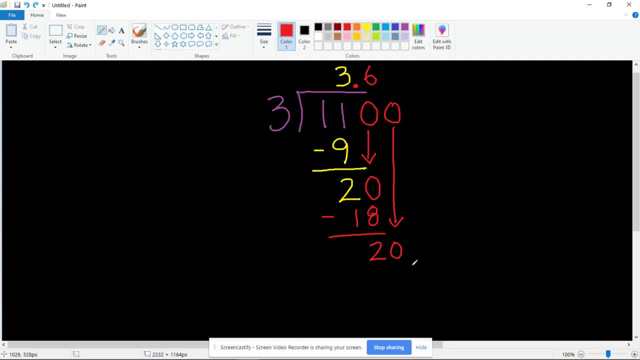 like we had here. It's going to keep repeating And once that happens we can do it one more time. Let's put a six in here: Six times three, 18.. Still two. See how this part is exactly the same. 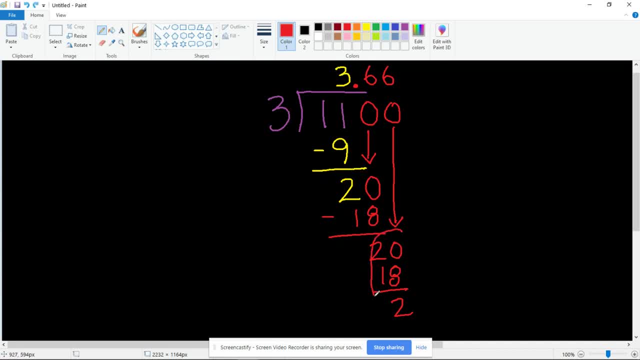 So this here is identical to this part right here. So once you get the answer, all you do is you give it a little hat, Put a line over the top of the part that repeats: So the answer would be three decimal six six. 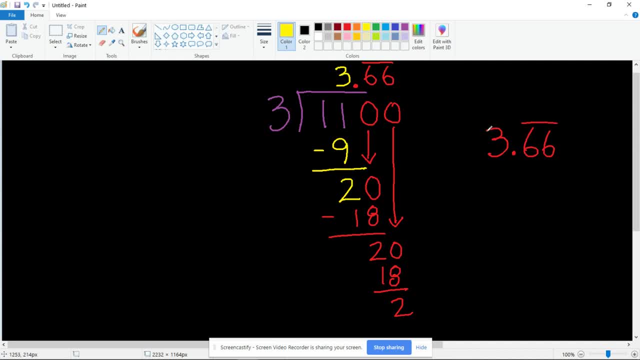 And if you get really fancy, you can look at this six here and know that let's change the color to white. The six here is closer to 10. So that's bringing in your rounding skills. Six is closer to 10. So that means this digit, the 10th, goes up by one. So you could also put 3.67.. And sorry.